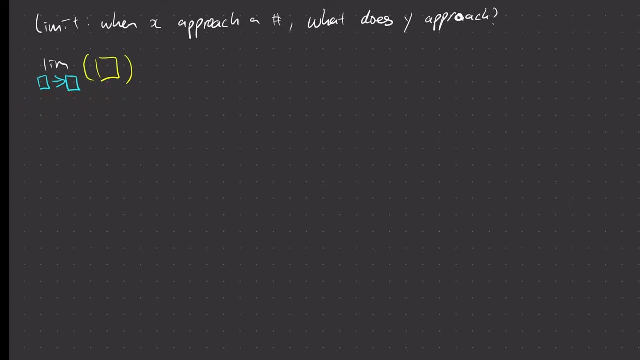 Very simple. So let me give you an example. Let's pretend we have f of x. We have a function: f of x equals x, squared right. The question could be like: oh, when x approaches 1,, what does y approach? okay? 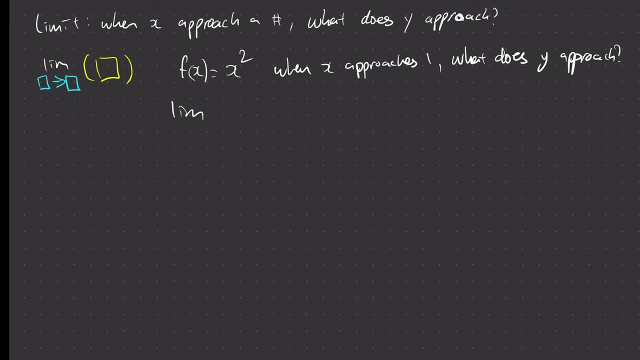 So how do you solve this? is we have to use limits, right? So we would do LIM like this, and then this here will be x, and then this will be 1, okay, So now, how do I know this is 1?? 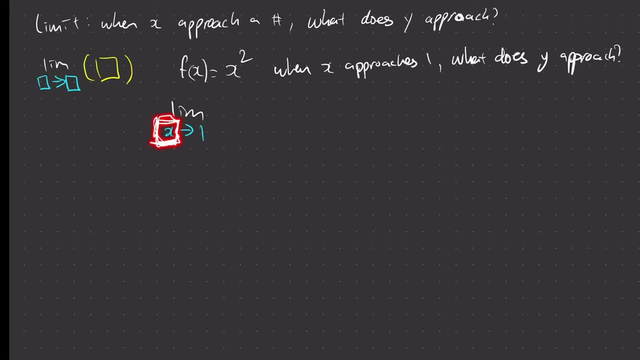 Sorry, how do I know this is x? okay, I know this is x because this is x here. okay, So this goes into here. Maybe I put an arrow like this, like this, And then how do I know this here is 1?. 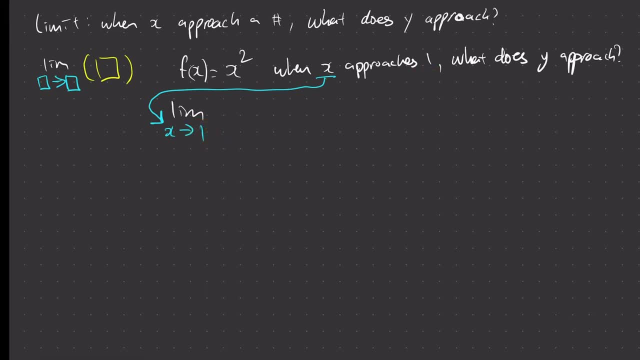 Because this one here is 1.. So I literally just here copy: number here, okay. And then what I put into the brackets. I put the brackets: this number, This here, okay, Like this. okay, Easy, No brain needed. 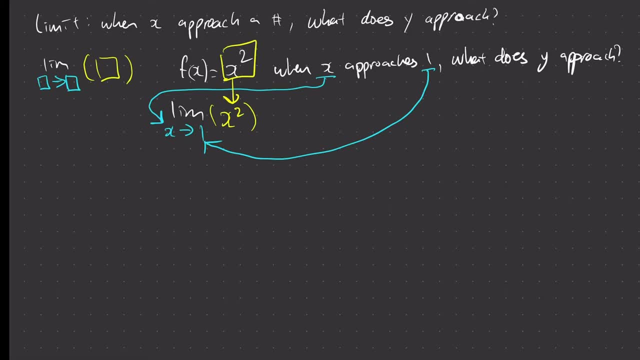 Literally just copy and paste the numbers. okay, No brain needed, And then what's next? Next is: what's next is: whenever you see x inside the brackets, you fill it in with the number 1, okay, How do I know it's x? 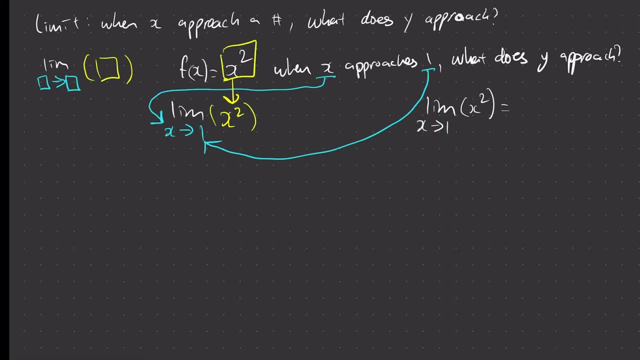 Because so this is x, right? This first letter, this first letter here, tells us to what to look for in the brackets. This tells us what to look for, okay, So I'm looking for x in the brackets, Okay, Okay. 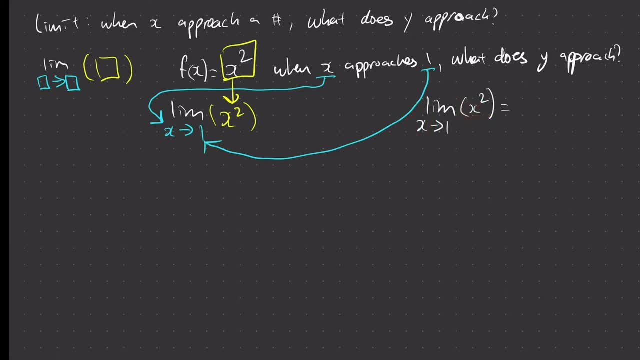 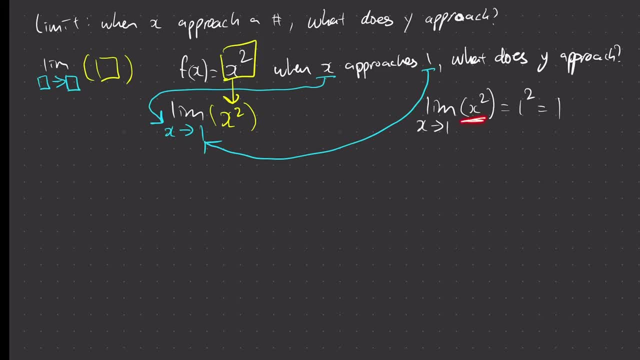 So the answer is just simply 1.. So when we know that for x squared, when x approaches 1, we get to 1, okay. Now let's say a more complicated question. So let's say we have f of x is equals to 2x squared plus 1, okay. 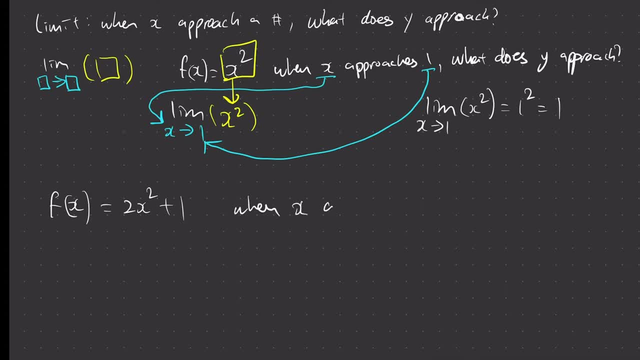 Again, when x approaches, Let's say number 2. What does y approach? Okay, So what does y approach? Very simple, Just no brain needed. the first step right, Just copy down all the numbers first. No brain needed. 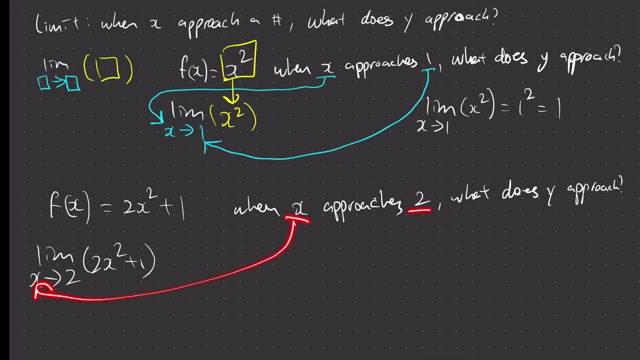 Copy down everything you need to do: X goes here, This goes here. This goes here. No brain- okay, And then what's next? Okay, So let's look at here What to look for. X- okay, I found my x. 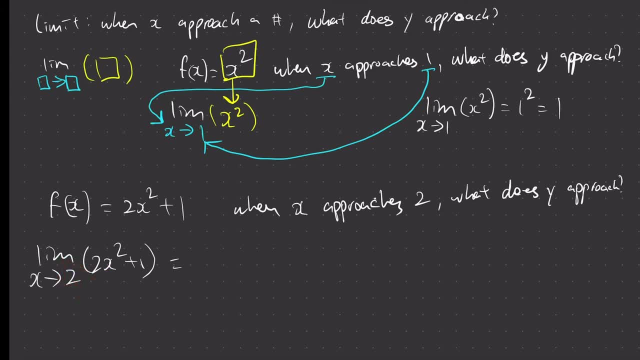 And then what do I sub it with? Sub it with 2, okay. So 2 squared plus 1,, which is 4 times 2, is 8,. 8 plus 1 is 9.. Answer is 9, okay. 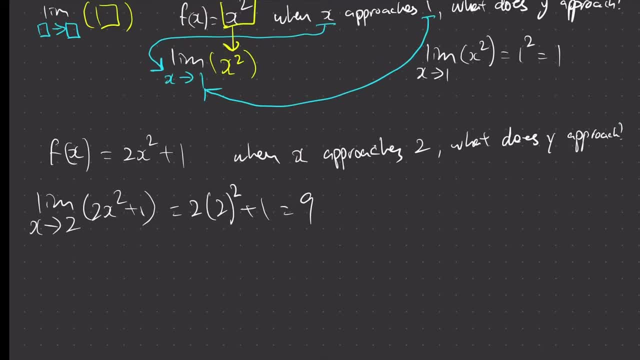 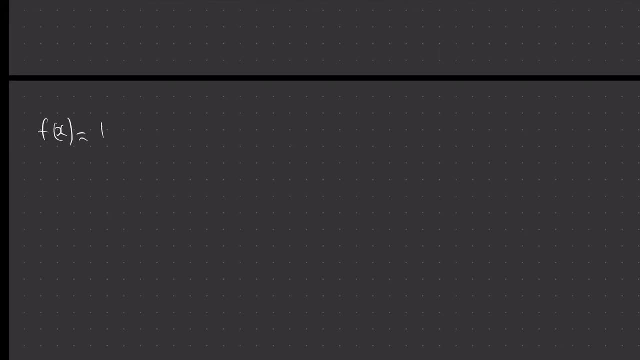 Just like that. Very easy, okay. Now even harder question: okay. So let's say we have f of x is equals to 1 plus e negative x, And we have g of x, It's equals to 2x plus b. okay, 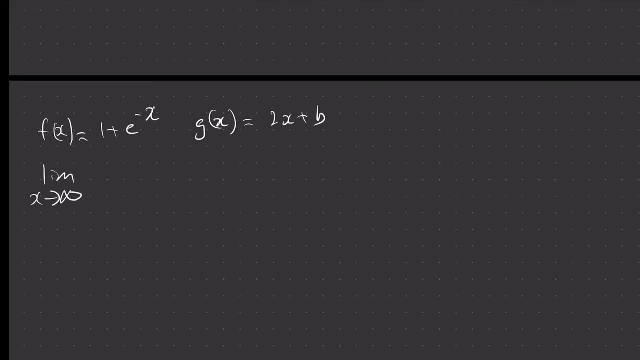 Now I want to find the limit of x to power. positive infinity of f, of g, of f, of x is equals to negative 3.. So right now is: we know when x approaches infinity? We know that when x approaches infinity we'll get to negative 3, right? 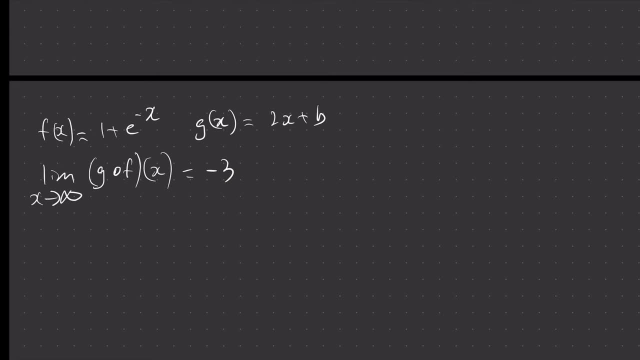 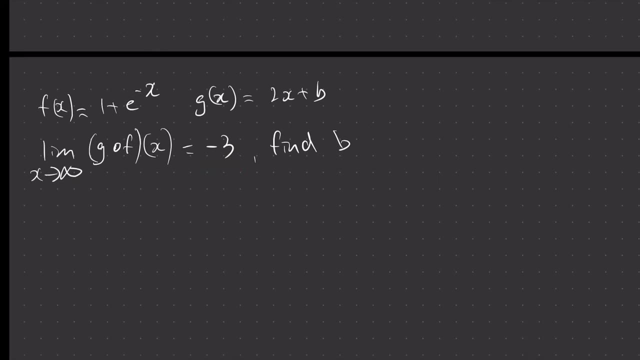 Okay, Negative 3.. But the question is asking you to find b. okay, So we know the limit is negative 3.. How do you do this? First is we obviously have to figure what this out, right? Figure this out. 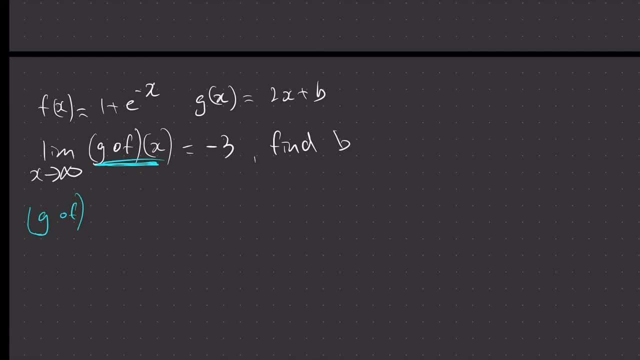 So we need to figure out this chunk. So we know that g of f of x is equals to put f into g, Put f into g. So we have this okay. Simplified is 2 plus 2e negative, x plus b. okay. 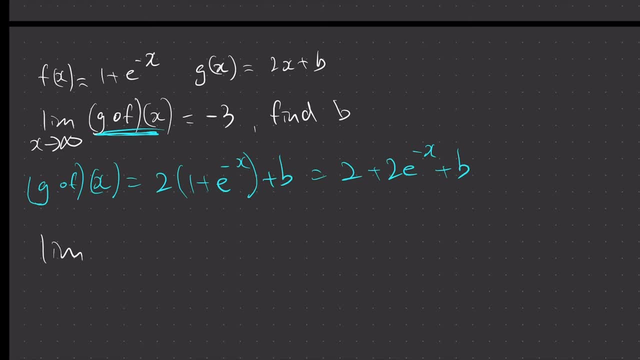 So now we have to put the blue stuff back into the chunk here, right? So then we have limit x. oops, x goes to infinity. open bracket: 2 plus 2e negative x plus b equals negative 3, right. 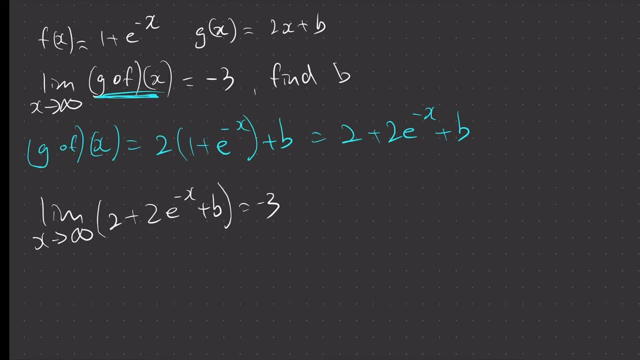 Okay, Just copying Again. no brain in this step. Brain is only needed for this step because there's expansion right And composite function. hope you guys already know that. Now what's next? Very simple, This letter here. this letter is x okay. 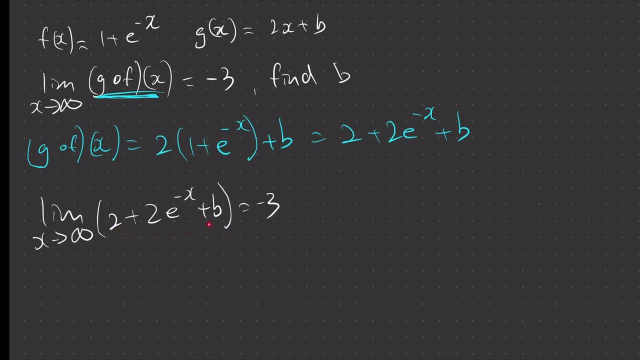 So that is the letter I'm looking for in the brackets, right? Okay, I have b here, not the number, not the letter I'm looking for. e here, not the letter I'm looking for. I have x here, x is the letter I'm looking for. 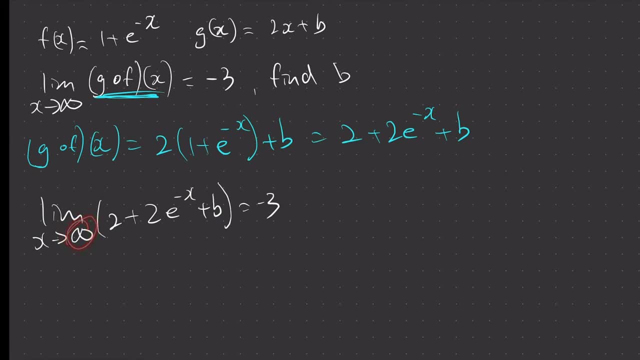 And what do I replace this x with? I replace this x with this number here, which is infinity. okay, So we'll have 2 plus 2e. negative infinity plus b equals negative 3, right Now, how do you look for b? 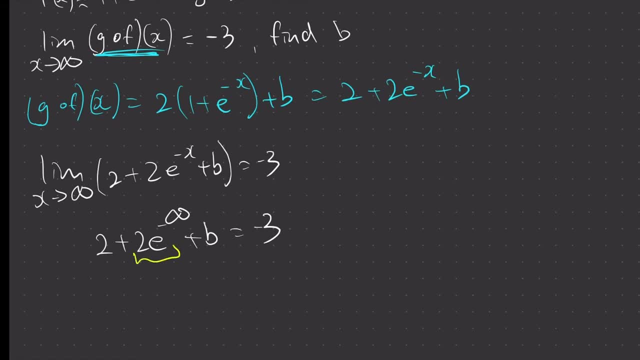 Well, have to use some brain here. We know this. here is basically 0. Why is this basically 0?? Because, according to exponent rules, we have a negative here, right? What does exponent rule tell us? When we have negative, we can rewrite it as 1 over e to the power of negative infinity. 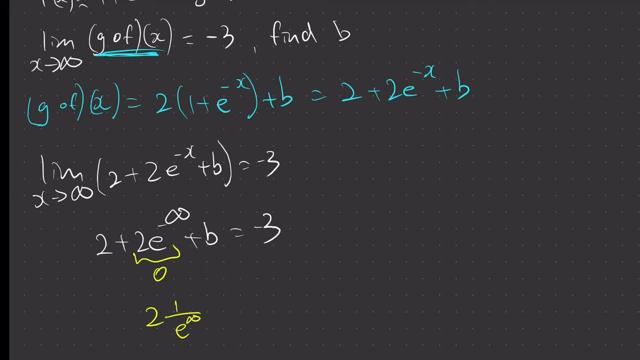 right, So this yellow thing can be written as 2, 1 over e to the power of positive infinity. Now we know that the bottom here is a very big number, right? If the bottom is very big, that means this entire fraction is very, very small. 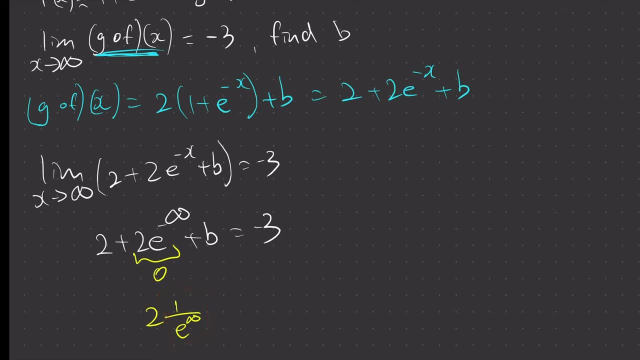 Very small, as in very close to 0. And we can pretend it's basically 0, right, 2 times 0 is 0. So we can basically ignore this. okay, We can pretend it's gone because it's very close to 0. 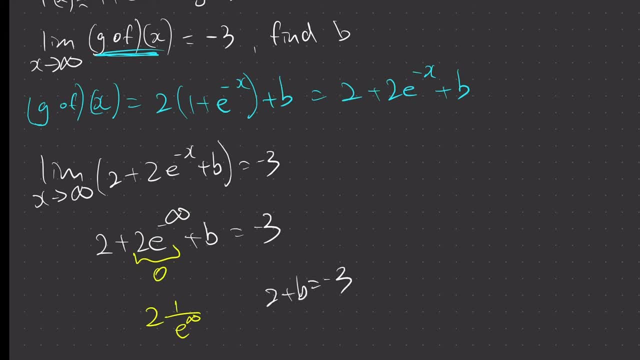 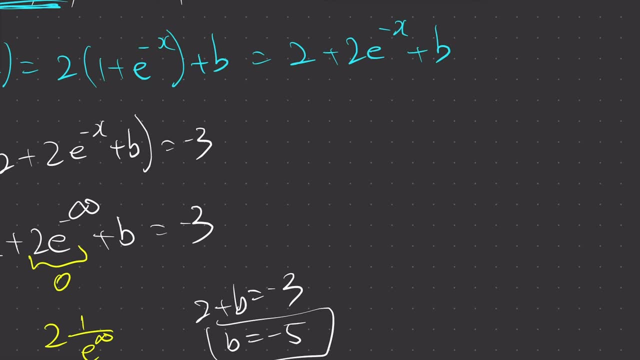 Now, if it's very close to 0, it's just 2 plus b is equal to negative 3, meaning b is equal to negative 5.. So this is your answer Done, Okay. So for homework or for practice, I'll give you a few more questions you can practice. 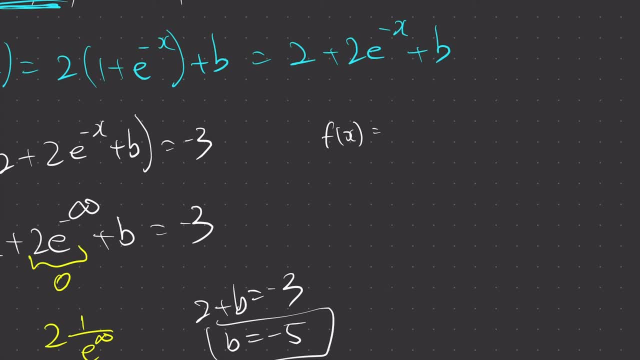 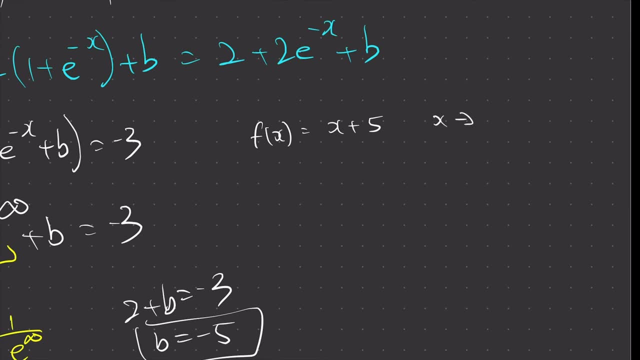 by yourself. Let's say f of x is equal to x plus 5.. And I want to find the limits of. let's say, when x approaches 2, what is y? Y equals what? Okay, So there's one question you can do. 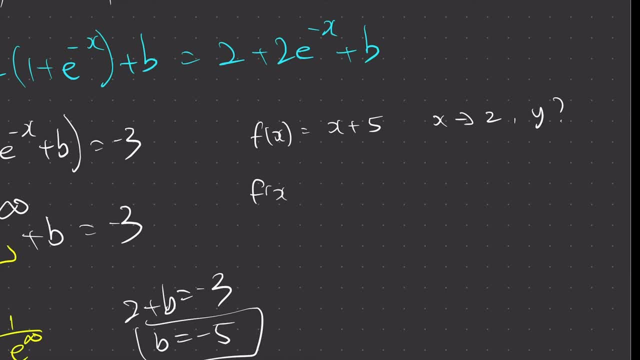 Very simple. Now, another simple question could be f of x. Okay, Okay, Okay, Okay, Okay, Okay. So f of x is equal to negative e, to the power of x, like this, And I want to say that if x approaches 5, what is y approaching? okay?